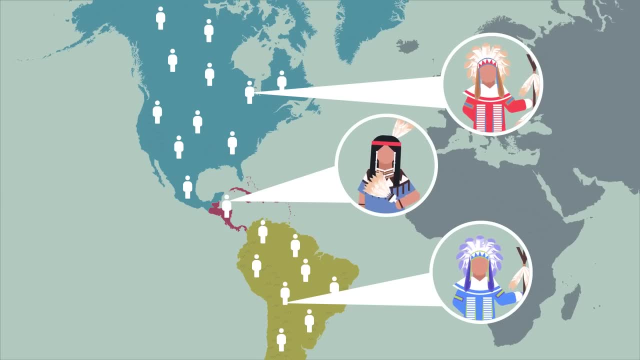 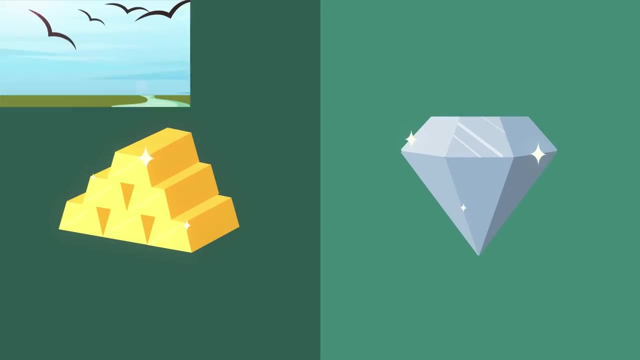 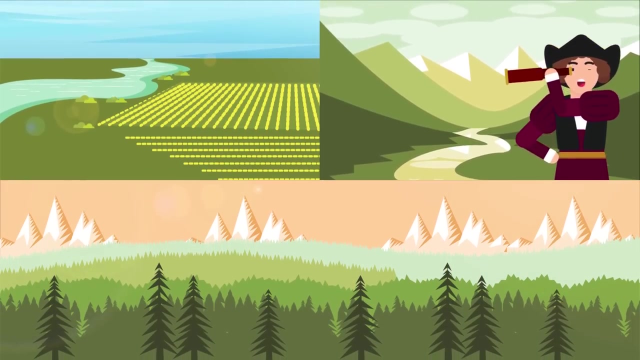 of native peoples that are now known collectively as American Indians or Native Americans, With great deposits of gold and other minerals, as well as vast plains, valleys and mountains. this new land was viewed by the Europeans as an enormous wilderness area with great economic potential, and thus became the land of dreams for those who were longing for resources. 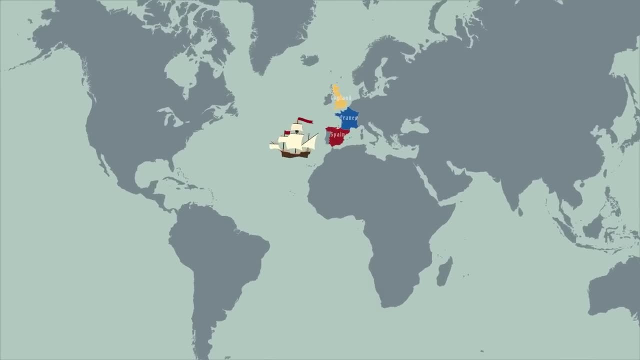 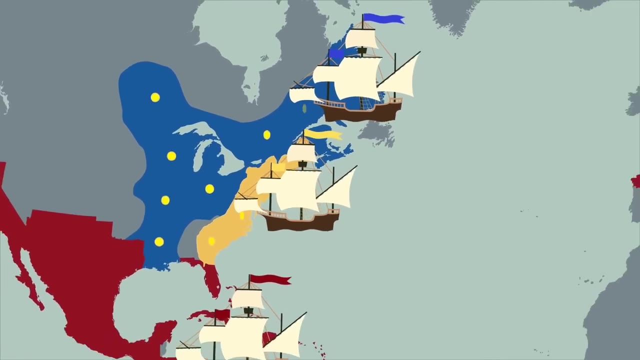 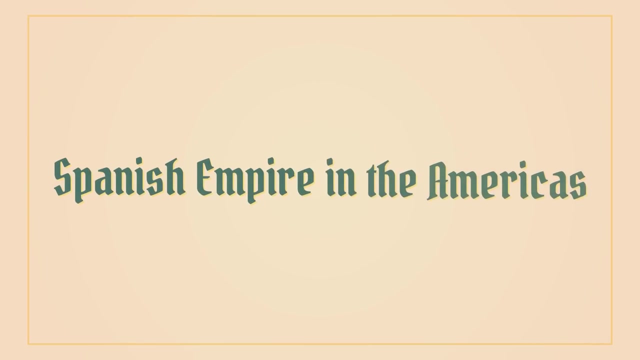 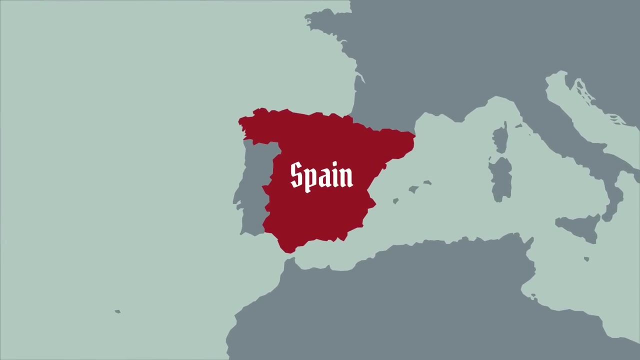 and wealth. This period of exploration and discovery soon became an international race of major European powers- Spain, France and England- to increase their wealth and establish colonies around the world. Spanish Empire in the Americas. The first European country to conquer and colonize the New World was Spain By 1512,. 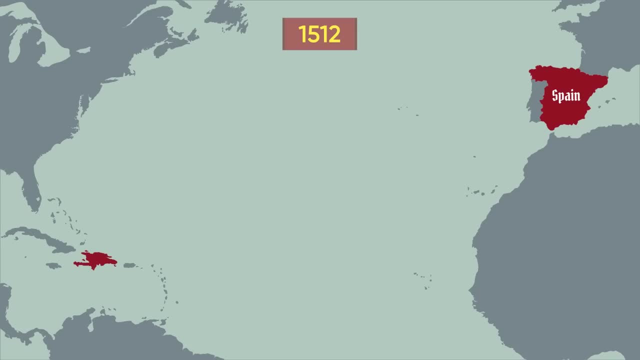 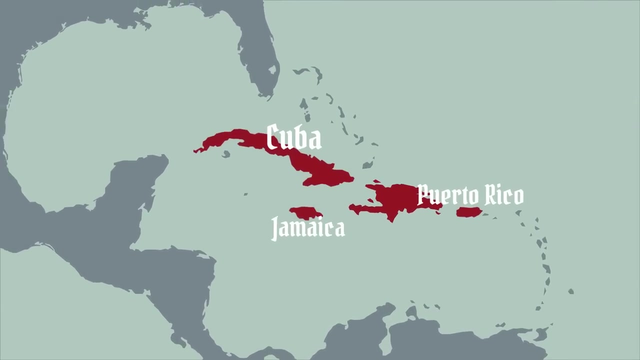 the larger Caribbean islands were occupied by the Spanish, with the first Spanish town established on the island of Hispaniola and Santo Domingo becoming the first capital of Spain's New World possessions. Other areas then settled by the Spanish were Cuba, Puerto Rico and Jamaica. Spanish conquistadors then sailed from the island harbors to explore. 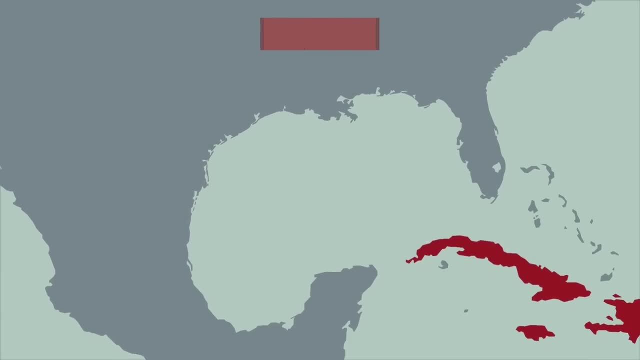 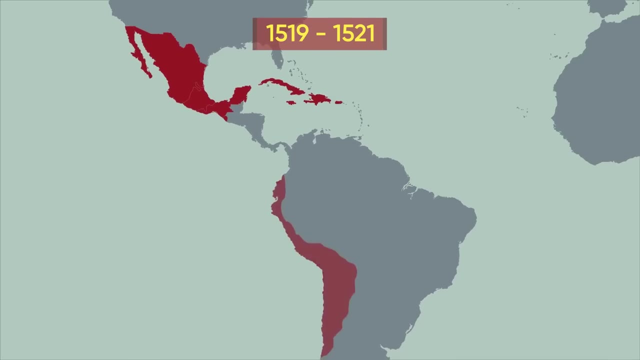 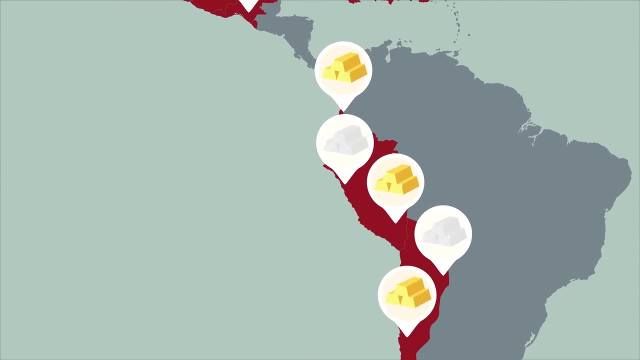 the coasts and penetrate the continents. In 1519 to 1521, they conquered the Aztec Empire in Mexico and a few years later took control of the Inca Empire and Peru. After growing rich from vast deposits of gold and silver in Mexico and Peru, Spain organized further. 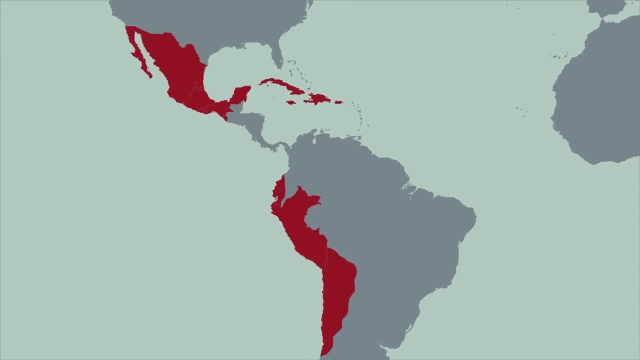 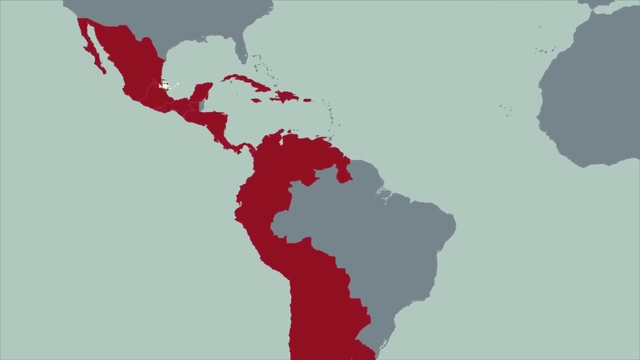 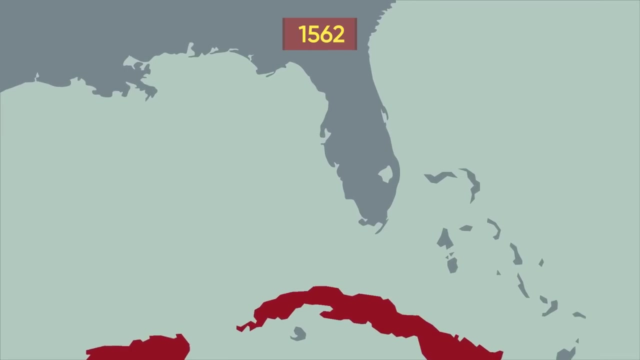 expeditions to the surrounding areas and soon settled most of Central America and South America, except for Brazil, which was colonized by the Portuguese. Other conquistadors ventured north into the southern parts of what is now the United States. In 1562, Northern Florida was settled by a group of French Protestants, Huguenots, forcing the Spanish to launch an expedition led by the Spanish. The Spanish were forced to leave the country and move to the southern part of the United States, where they were then forced to leave. The Spanish were then forced to spy on the Spanish and from Mexico they leadership. 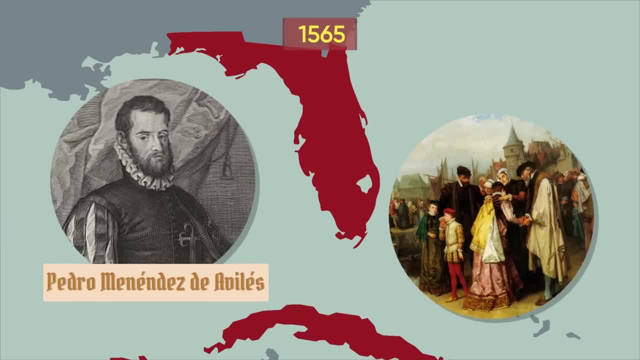 a large 제일 at the mouth of another Spanish colony called the Monasterio de Santa Fe, which was now known as the Monasterio de Santa Fe. This colonization continued until a Spanish invasion of Mexico's port was created by the explorer Pedro Menendez de Aviles in. 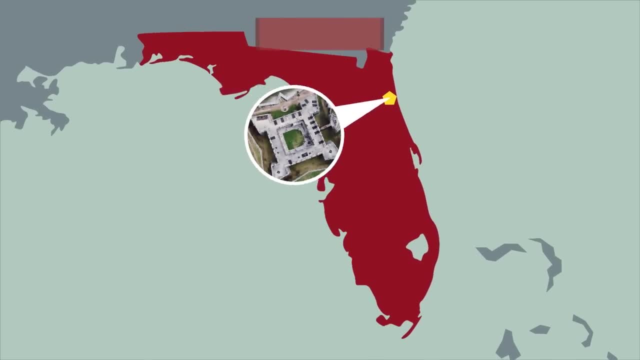 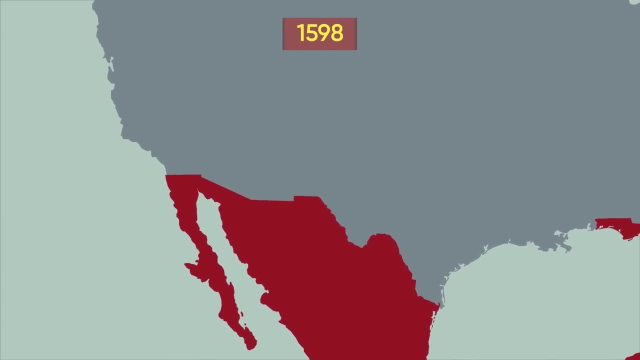 1565.. Most of the French colonists were killed and a Spanish fort was built on the site of what is now St Augustine. Later, in the 16th century, Spain began colonizing the region north of Mexico. In 1598, a group of Spanish settlers arrived in the New Mexico-Arizona. 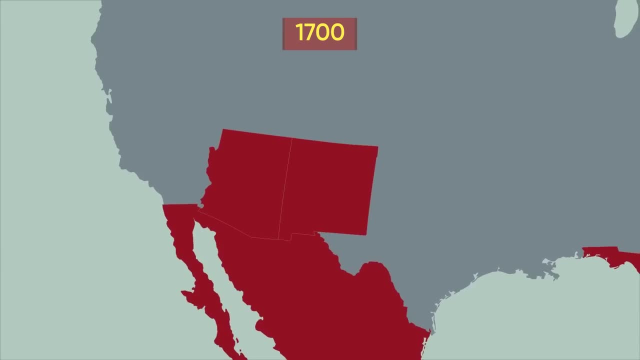 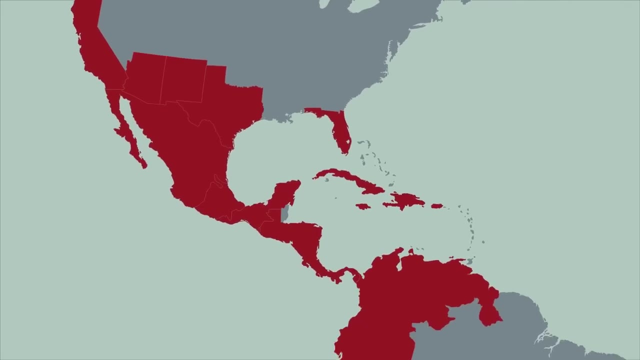 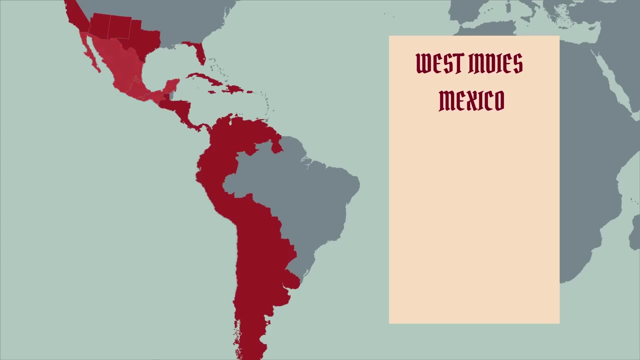 area and the city of Santa Fe was founded in 1610.. managed to colonize other outposts in North America, Texas and California. After all, Spain possessed the largest land area of the colonial empires in the New World, including several islands in the West Indies, all of Mexico, most of 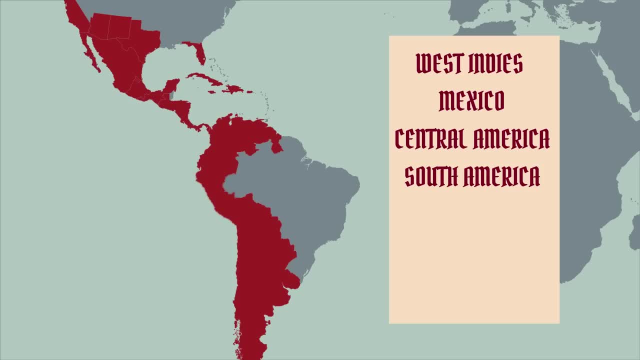 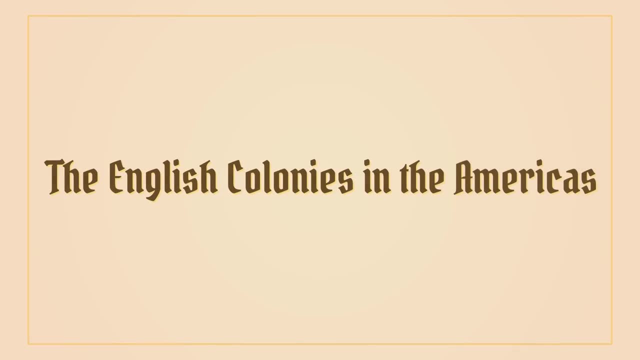 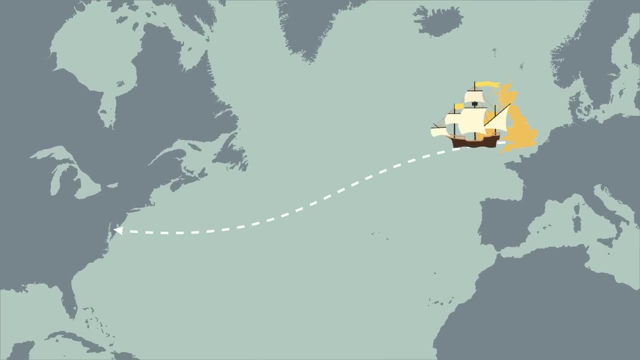 Central America, most of South America and what are now Florida, California and the US Southwest, The English Colonies in the Americas. England also took part in the exploration and colonization of the Americas and their most significant establishment proved to be the Thirteen Colonies along North America's Atlantic. 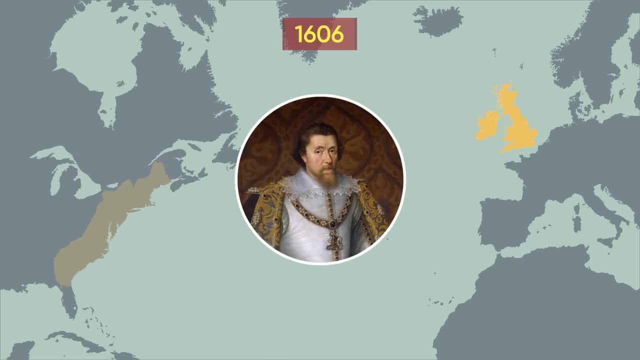 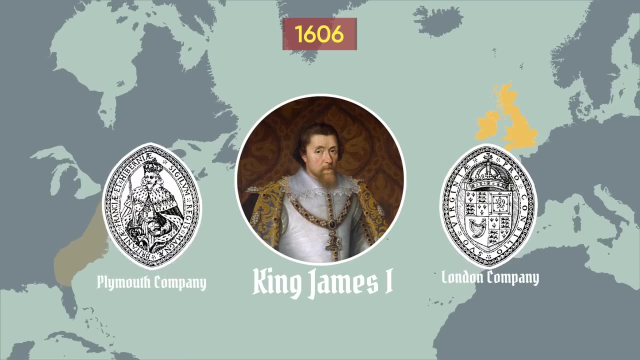 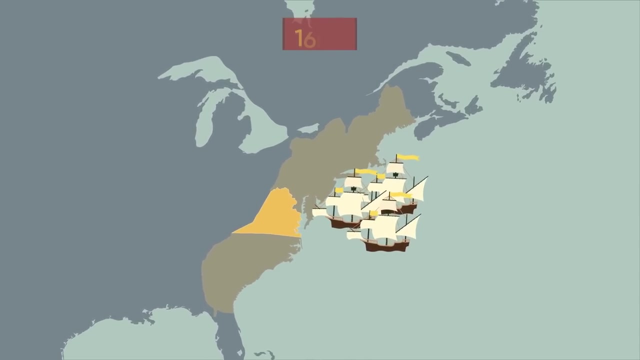 coastline. In 1606,, just a few months after King James, I granted charters to the London Company and the Plymouth Company to establish permanent colonial settlements in North America. three ships were sent by the London Company to what is now Virginia In 1607,. they reached the Chesapeake Bay and headed about 30 miles north of the Atlantic coastline. In 1607, they reached the Chesapeake Bay and headed about 30 miles north of the Atlantic coastline. In 1607, they reached the Chesapeake Bay and headed about 30 miles north of. 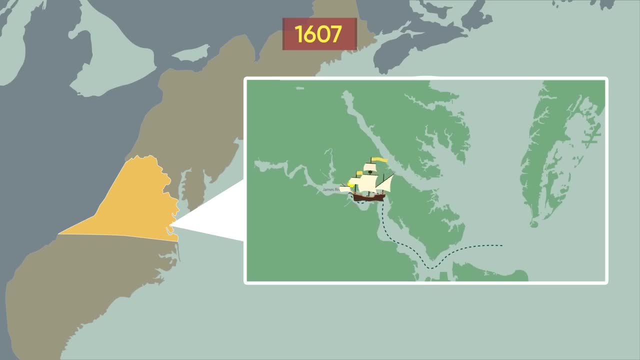 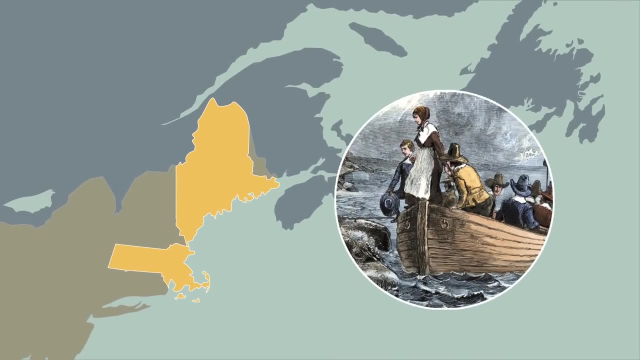 the Atlantic coastline In 1607, they reached the Chesapeake Bay and headed about 60 miles up the James River where they built the first permanent colony called Jamestown. The second successful English settlement in America was the Plymouth Colony in what is now Massachusetts in 1620 by the Pilgrims. 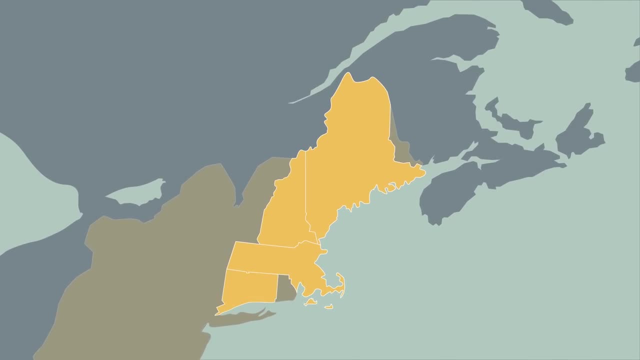 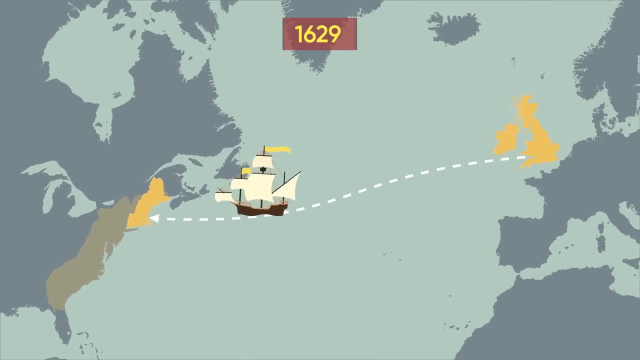 Following the success of the Jamestown and Plymouth colonies, colonies were gradually established by the English in the region that became known as New England Massachusetts Bay. another settlement established in 1629, was the landing place of the Mayflower and the Pilgrims. As Massachusetts prospered and expanded, the settlers sought the new colonies in New England. New Hampshire was another piece of New England to be formed in 1632, Connecticut and Rhode Island were formed in 1635 and 1636 respectively for people to have the opportunity to live. 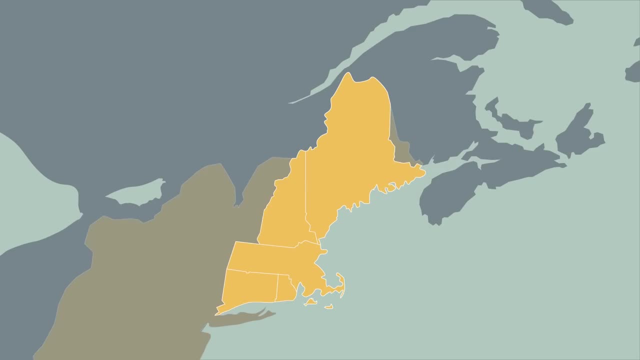 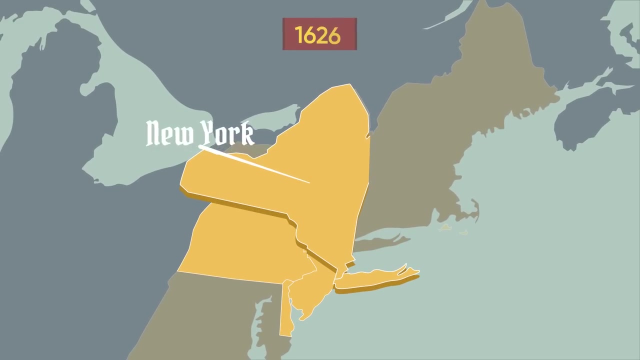 and worship in accordance with their beliefs. Today, New England also includes Maine and Vermont In the middle colonies. New York was originally colonized by the Dutch in 1626 with the name New Netherland, but then became the English colony in 1664.. 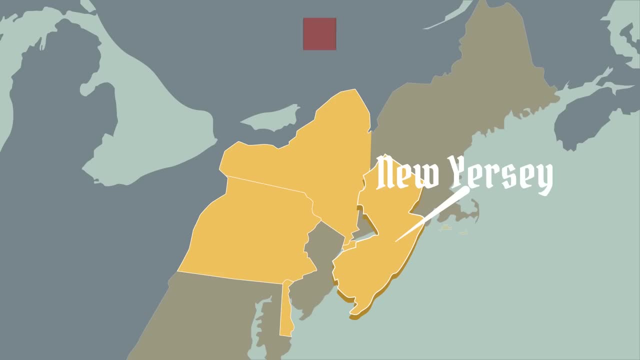 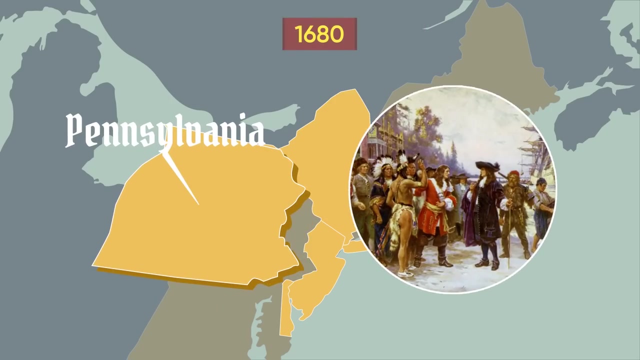 This colony also included the first permanent settlement in New Jersey. Delaware, as part of the Swedish colony in New Sweden, was founded in 1638, and then became an English colony in 1664.. In 1680, the Quakers settled Pennsylvania, forming the last piece of 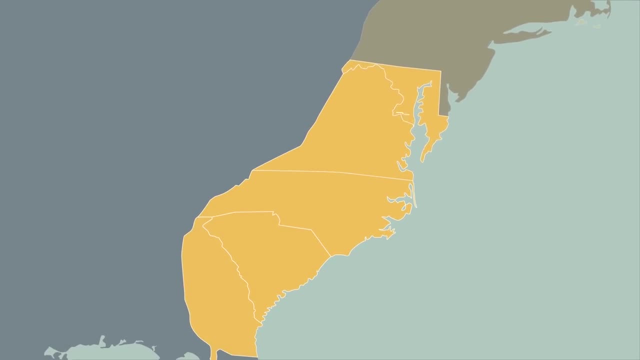 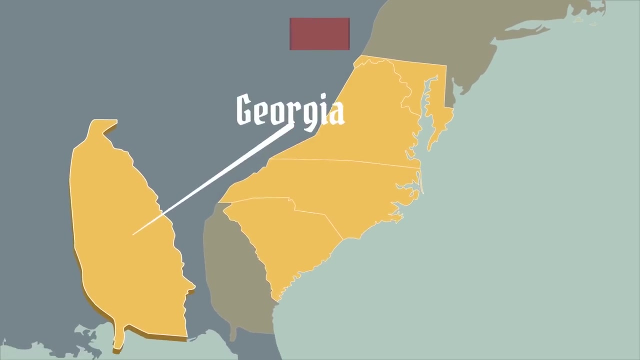 the middle colonies. In the southern colonies, the English settled Maryland to the north of Virginia in 1634 and Carolina in 1653, later split into North Carolina and South Carolina in 1729.. Georgia Colony was established in 1732 as a buffer zone between the British colonies. 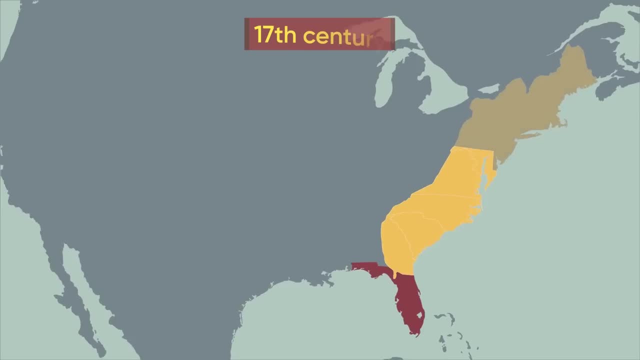 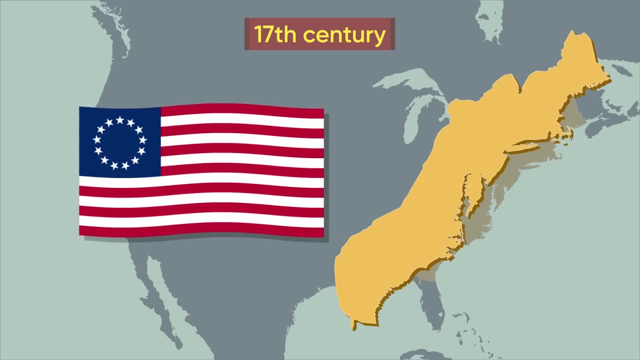 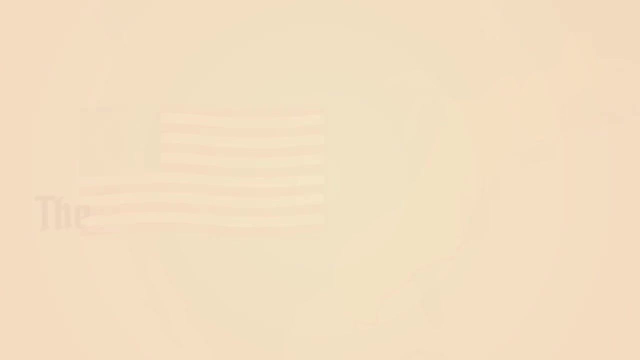 and Spanish settlements in Florida. By the 17th century, the English had taken the lead in colonizing North America, with the formation of the Thirteen Colonies which later became the Thirteen original states of the United States of America, The French Colonies In The Americas. 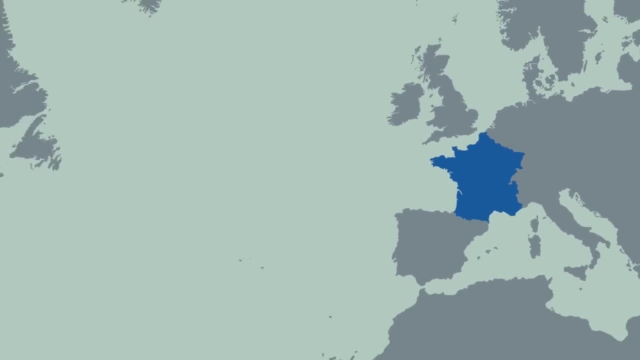 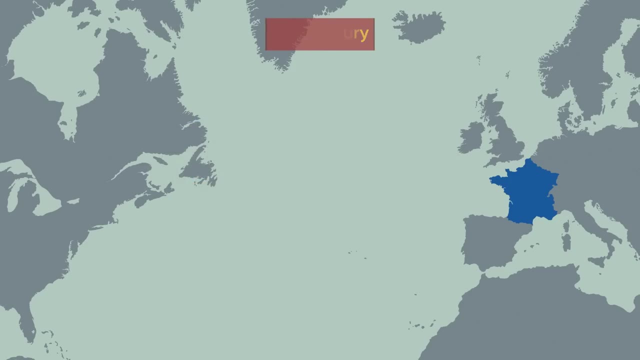 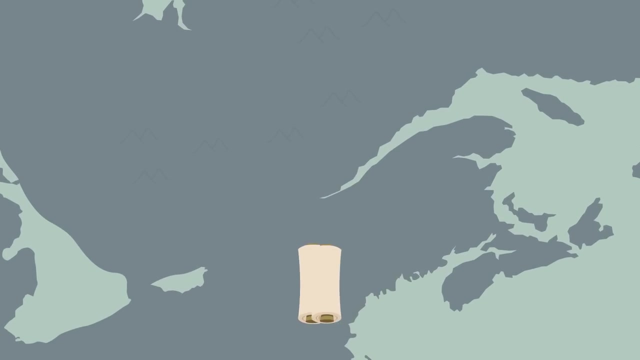 France, one of the two northern Atlantic kingdoms besides England, began sending ships to explore and colonize the Americas. in the 17th century, In North America, France established a large colony called New England- New France, Seeing the potential for fur trading. the founder of Quebec in 1608, Samuel de Champlain. 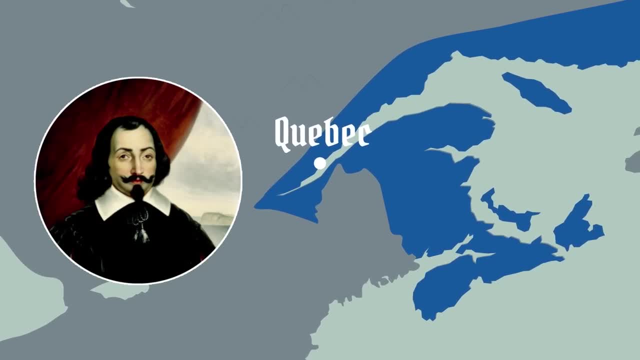 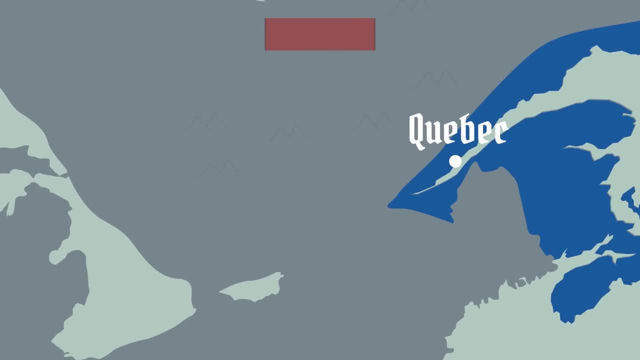 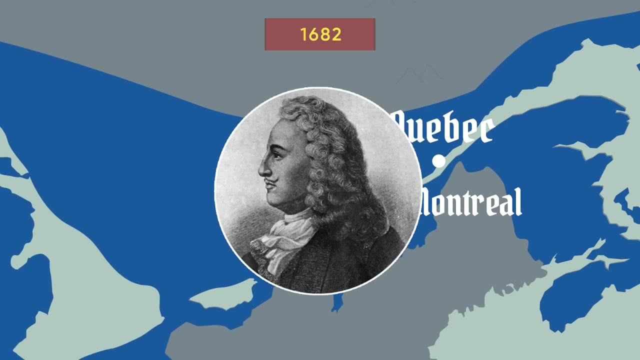 attempted to explore the region and to build up the French fur trade with the help of the Huron Indians. Three years later, he established the beginning of a settlement on Huron Island, which is today the site of Montreal. In 1682, René Robert Cavalier, the most famous of all, the 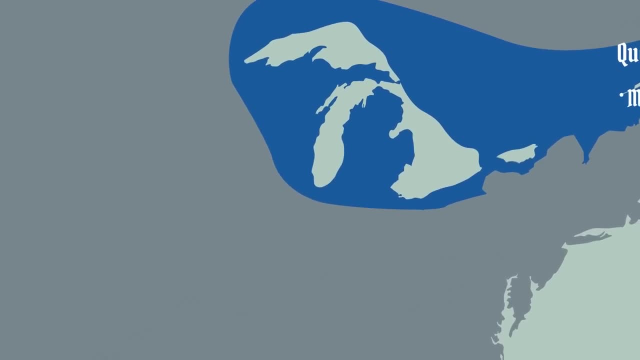 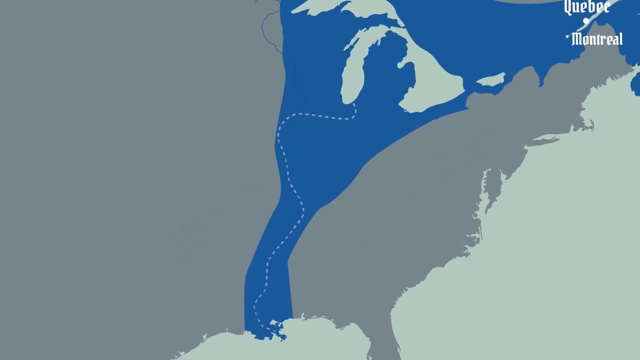 explorers had his expedition to send the Mississippi River from the Illinois Territory to the Gulf of Mexico and later claimed the entire territory for France. Many other French permanent settlements in North America were founded, including Detroit, St Louis, Baton Rouge. 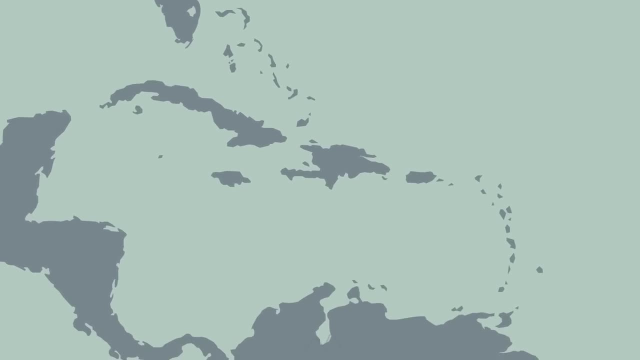 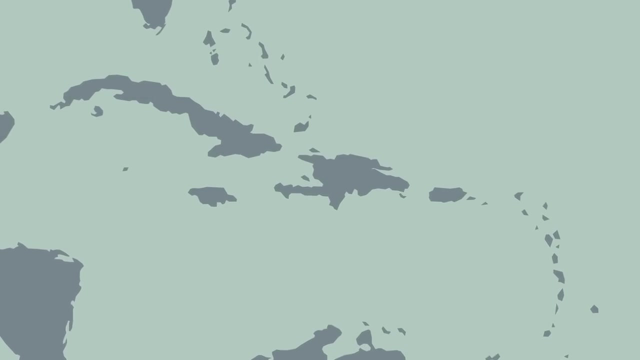 and New Orleans Down to the Caribbean islands in South America. by 1664,, France controlled 14 islands in the Caribbean, with the principal possessions including Saint-Domingue, now Haute-Marie and Saint-Domingue. In the late 16th century, France had the opportunity to 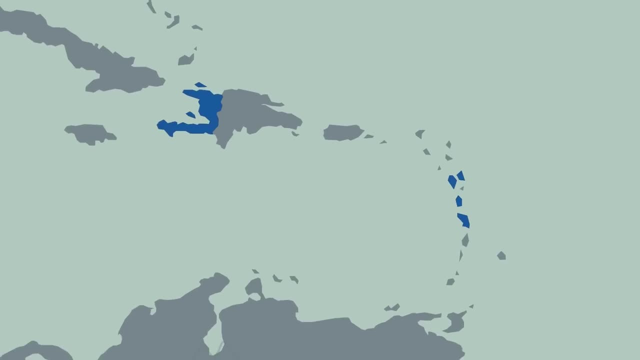 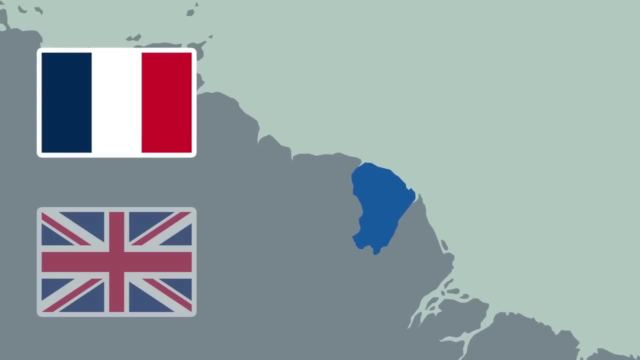 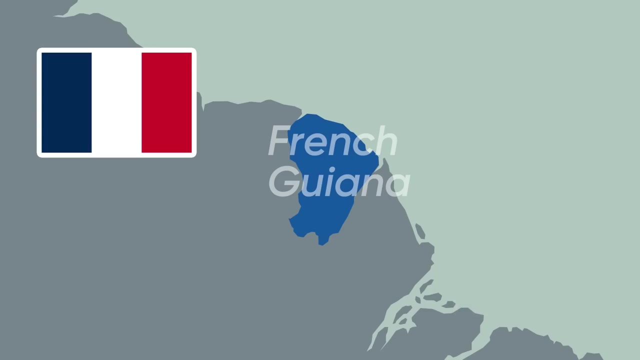 conquer Haiti, Martinique, Guadeloupe and Dominica On the northeast coast of South America. after numerous changes in control alternating between France, Britain, the Dutch, the Netherlands and Portugal, the colony of French Guiana was finally confirmed as French in 1817.. 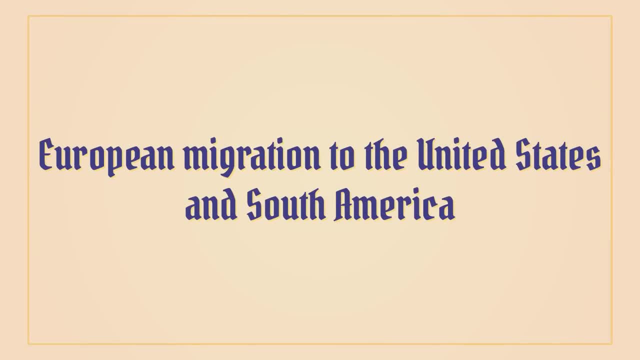 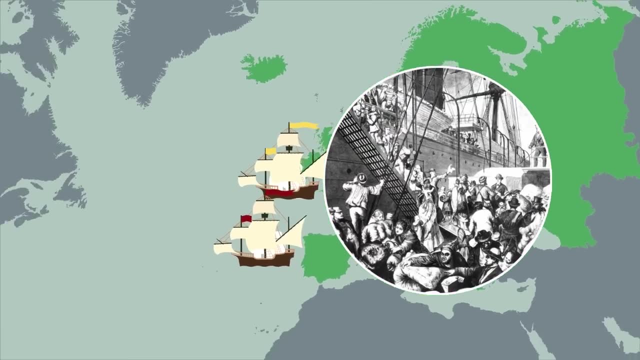 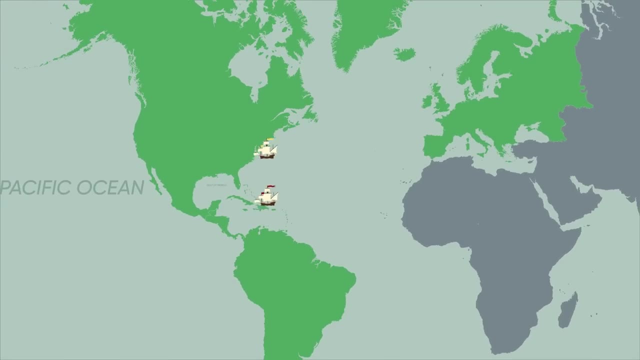 European Migration to the United States and South America. During the colonial era, millions of people left Europe and immigrated to the Americas, mostly in the United States and South America, seeking either economic opportunities or religious freedom. From 1815 to 1865,. 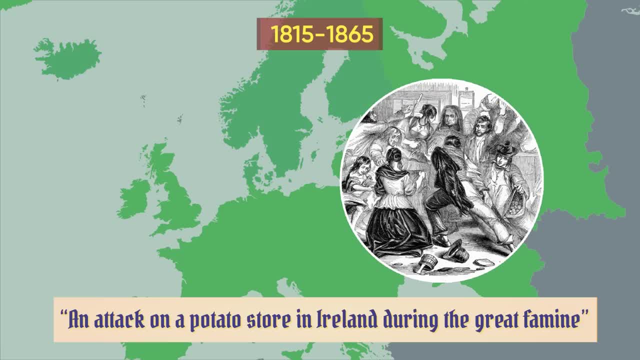 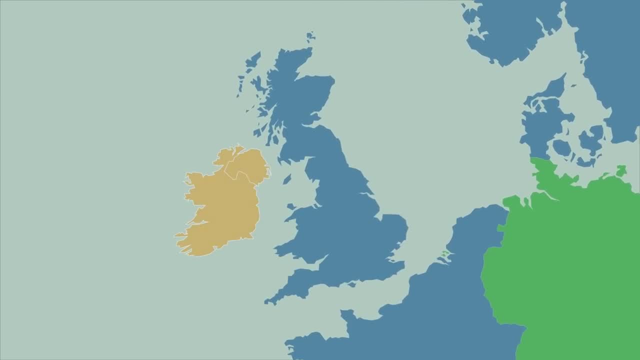 thousands of migrants sailed mainly from Northern and Western Europe to America due to crop failure. At that time all of Ireland was part of the UK and most of the migrants were Irish unskilled labor coming to America to avoid starvation Also. 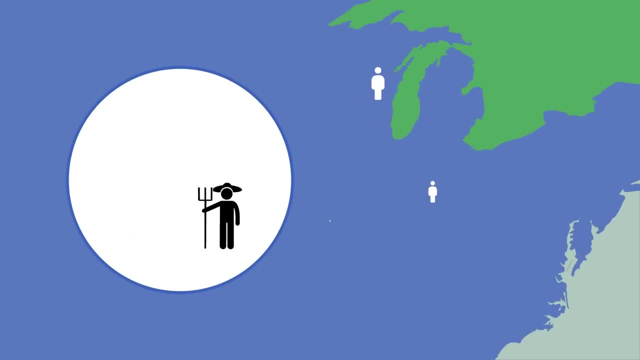 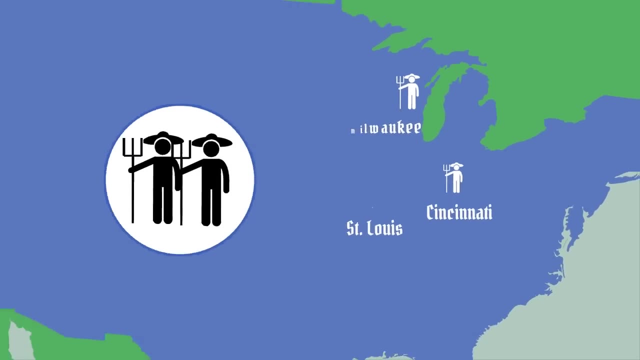 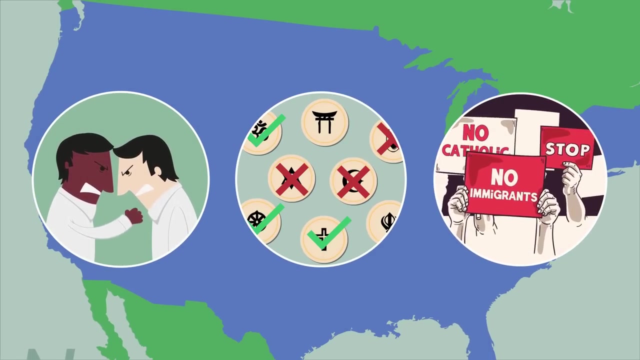 half of 5 million German coming to the US became former settlers in some areas that are now cities such as Milwaukee, St Louis and Cincinnati. The influx of immigrants resulted in competition for jobs, religious discrimination and protests across the country. In the 1850s, the anti-immigrant 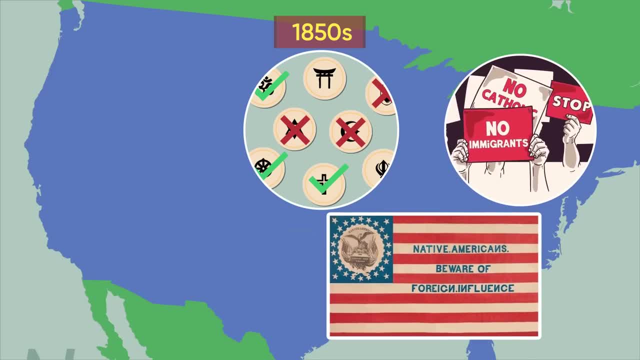 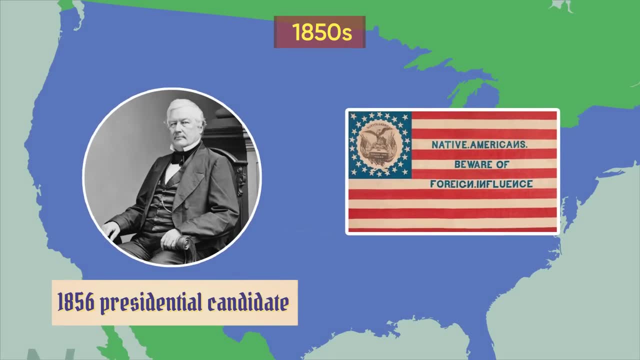 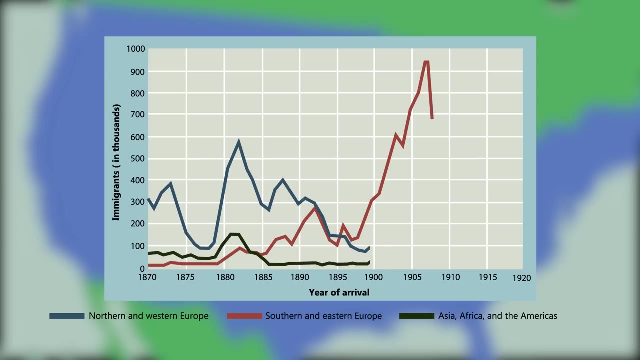 anti-Catholic American party, also called the Know-Nothings, attempted to put a curb on immigration and even won several governorships and legislative seats in the presidential election of 1856.. Following the Civil War, rapid industrialization and urbanization from 1880. 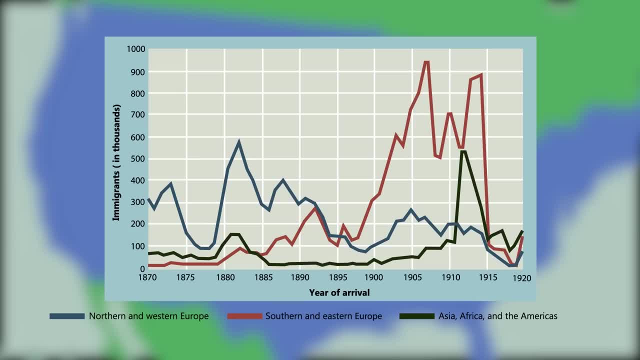 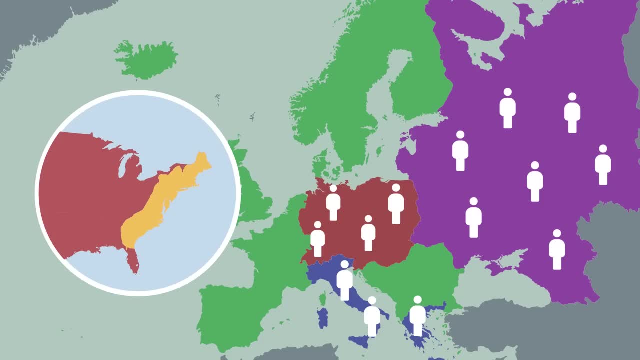 to 1920 made the immigration situation a bigger wave. The majority of more than 20 million immigrants were from Central, Eastern and Southern Europe, with different motivations, such as job opportunities and freedom of religion. In addition, many Africans were born and raised in the United States, and many of them were born and raised in the United States. 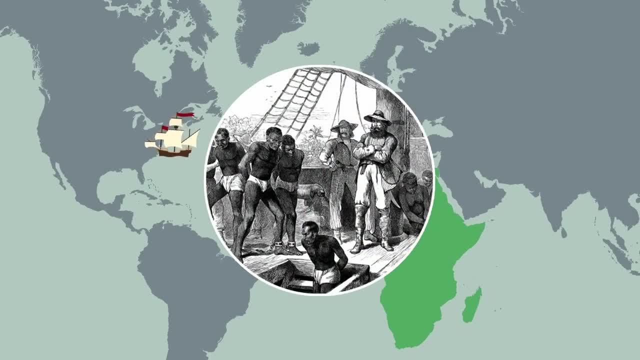 In addition, many Africans were born and raised in the United States, and many of them were born and raised in the United States, and many of them were born and raised in the United States, were brought to America and sold into slavery. The opium wars of the mid-19th century between: 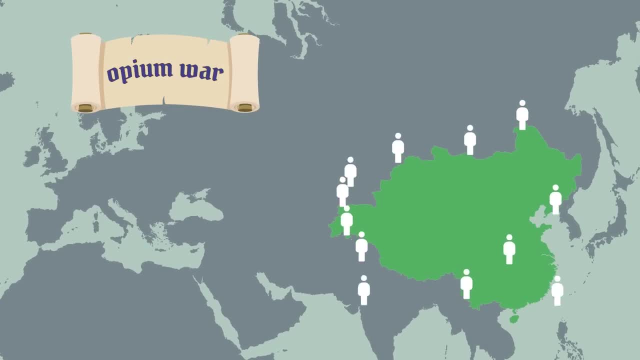 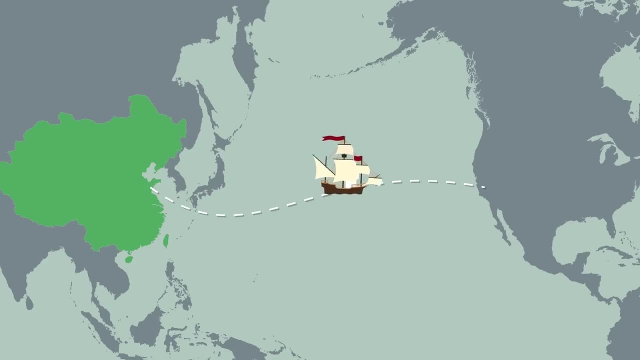 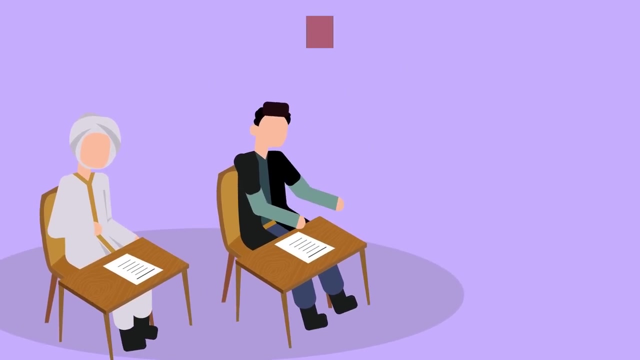 Great Britain and China put China in debt and many Chinese left the country to find work. As a result, Asian immigrants, mainly from China, crossed the Pacific to join the California Gold Rush, The flare-up of World War. I eased the trend of immigration.